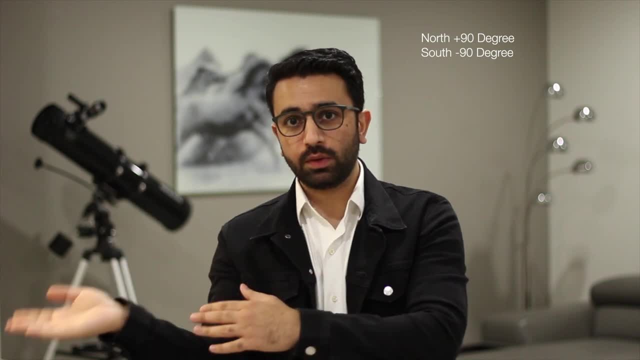 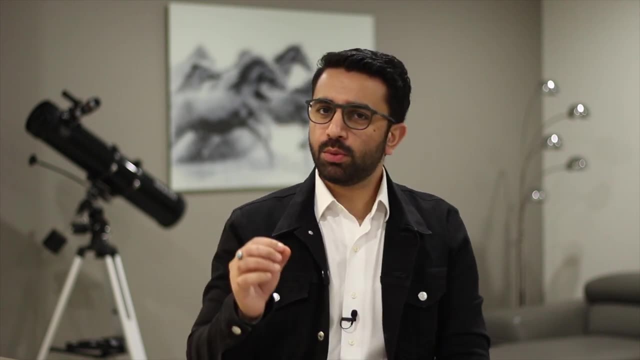 be positive 90 degrees and if you move it all the way down to the south, it would be negative 90 degrees. with the celestial sphere and using these coordinates of right ascension and declination, we can pinpoint the apparent positions of the stars in the night sky and note that this position 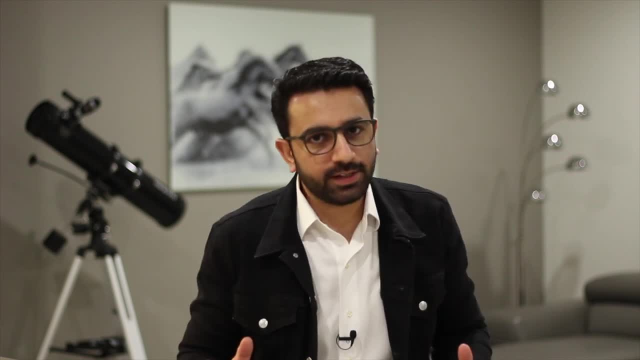 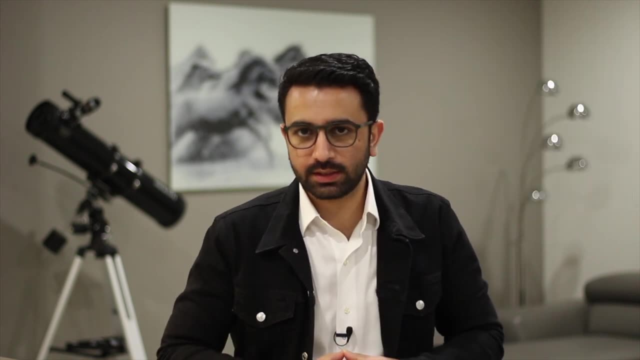 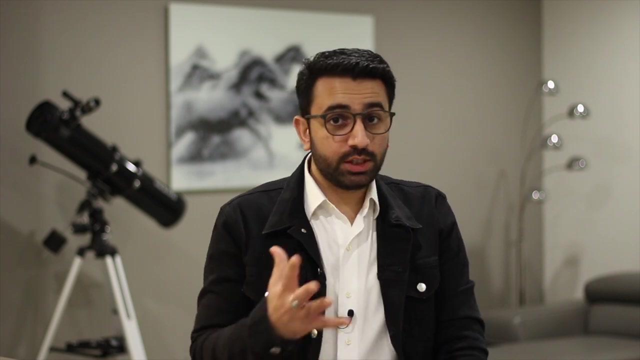 does not change over a period of time- okay, it does, which is due to earth's precession, and it takes over a period of 25,772 years. i know it's that long and if you calculate it, it's just over one degree over a whole century, which is pretty insignificant in a human's lifespan. and until 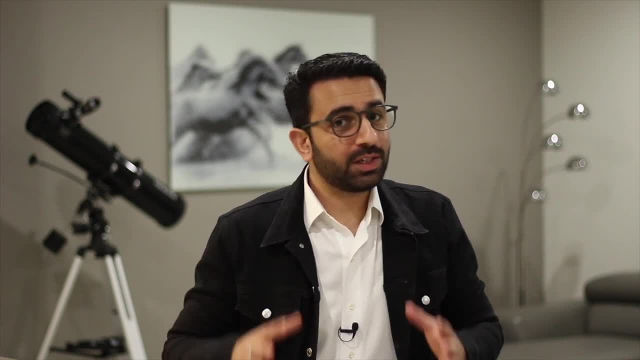 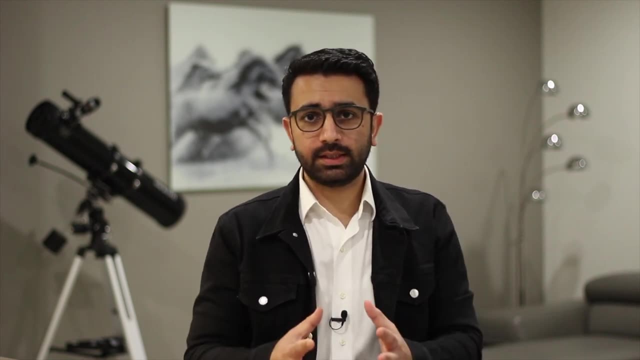 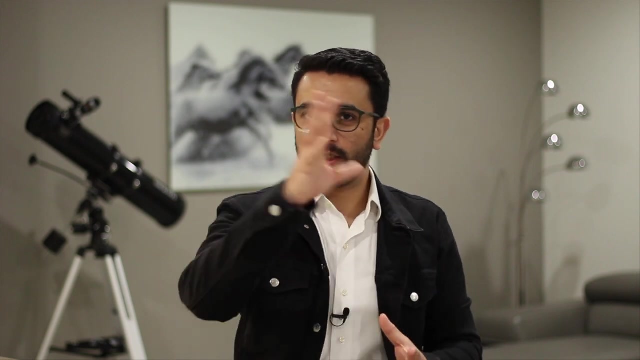 unless you're a scientist, you wouldn't really notice the difference. but not everything in the night sky changes its position over that long- for example sun planets and the moons- and it's because they keep on changing their position relative to each other and that's the reason why they kind of move differently through the sky. all right, so celestial. 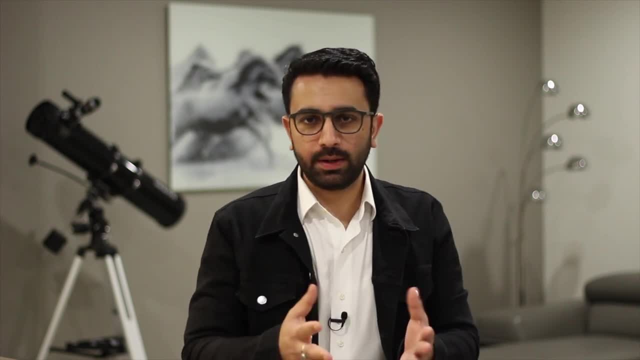 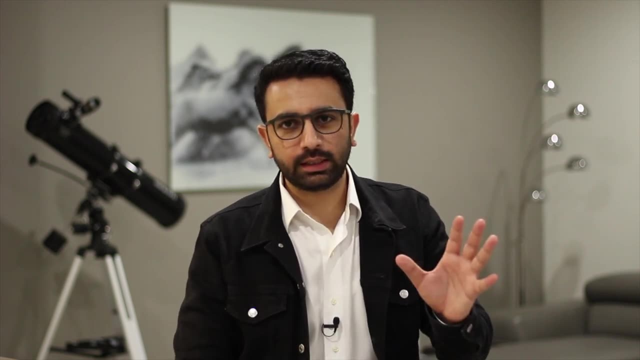 sphere coordinates are fixed, which means we can put it on a celestial map, and it's only going to get outdated after 26,000 years. anyone who knows these coordinates can easily go and find an object in the night sky or the day sky, and it's particularly useful if you're trying to find a 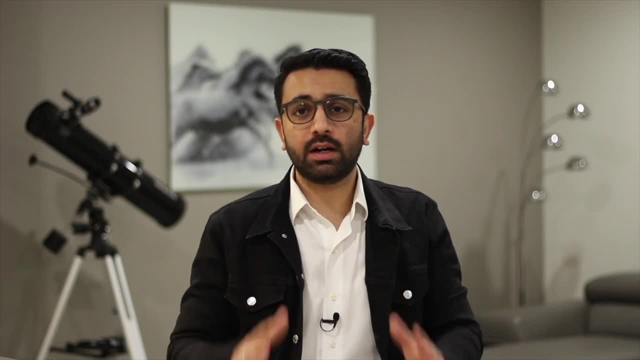 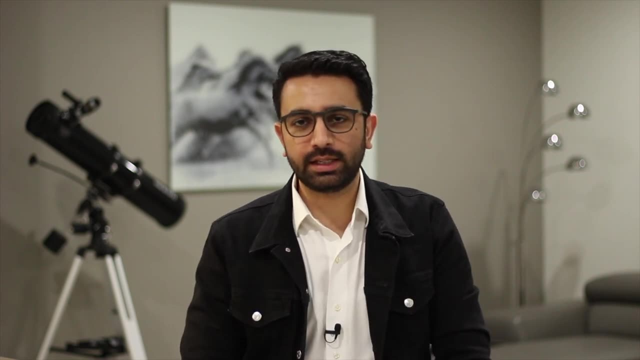 deep sky faint object which is otherwise very hard to locate. all right, with all that in mind, coming back to the point of how to use the ra and deck setting circles on the telescope, we need to start by polar aligning the telescope and notice when you point. 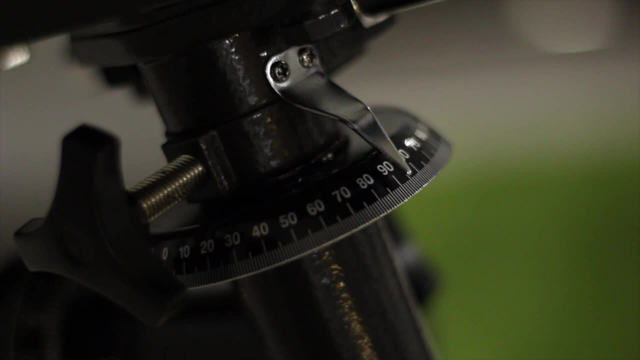 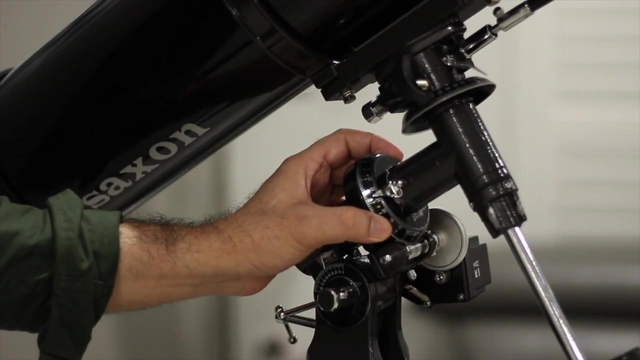 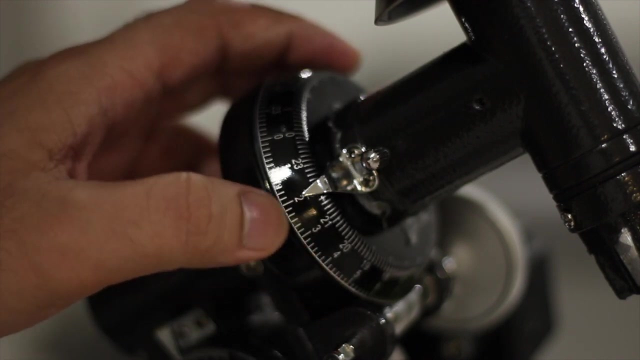 your telescope towards north or south celestial pole. the declination would say positive or negative, 90 degrees, just as we learned. now you need to set the ra dial. you can either look up the ra coordinates from google or any of the free apps like stellarium for north or south polaris, whichever, 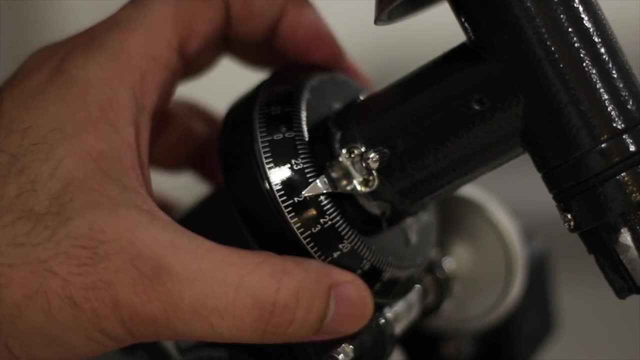 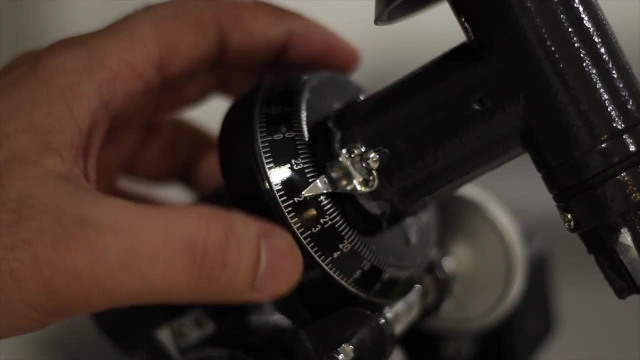 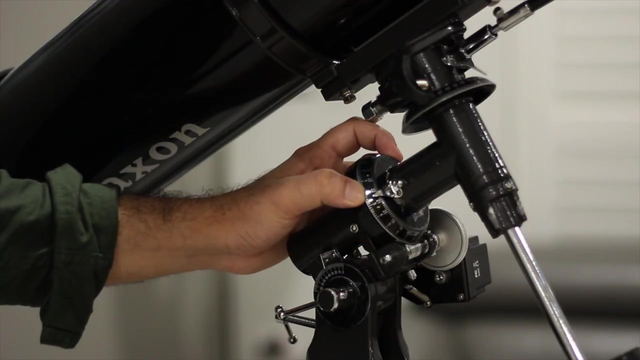 the one you're observing, and notice that the dial has 1 to 24 numbers, every one of which represents an hour, and on my telescope every hour is spread in six part, which means it's divided in 10 minutes each. so let's rotate the ra setting circles to match the ra of the star in the viewfinder and voila, we're ready.